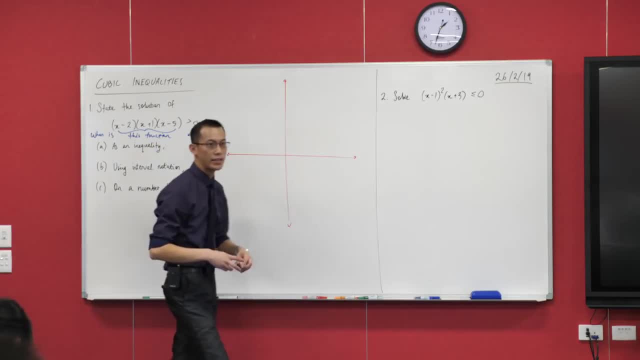 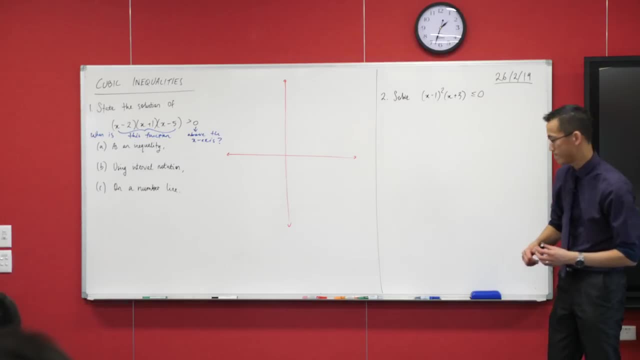 It's in a nice neat factorized form, so we should be able to really quickly read off the x-intercepts, right? How do you read them off? How do you use the factorized form? Any takers? Think, think, think, guys, this is this morning, right. 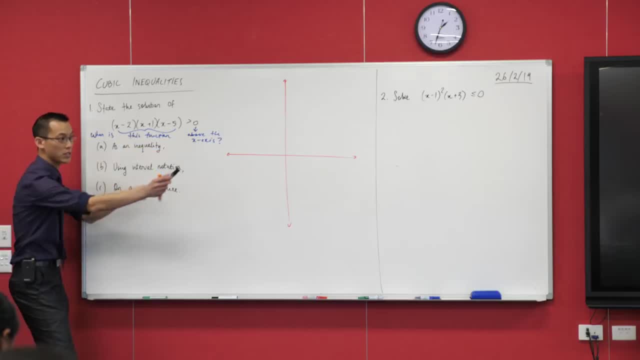 I should be able to read a solution from each factor, right? What's the first one? Two, just before you go on, I'm getting two from this guy here, right? If I were to put x equals two into here, the whole thing would become zero, right? 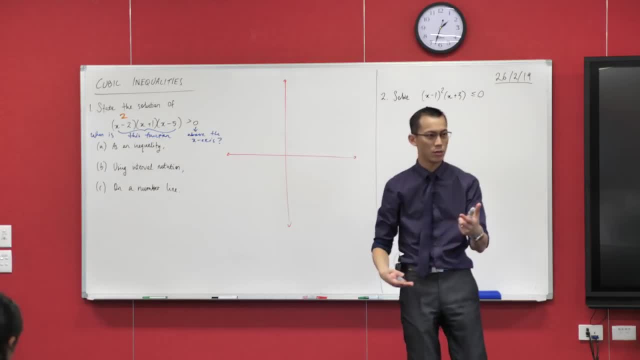 So that gives me an x-intercept right. You can then read off what the other ones are. The next one, Rishan, Negative one. very good, If I put negative one into here, all the rest of it becomes zero. 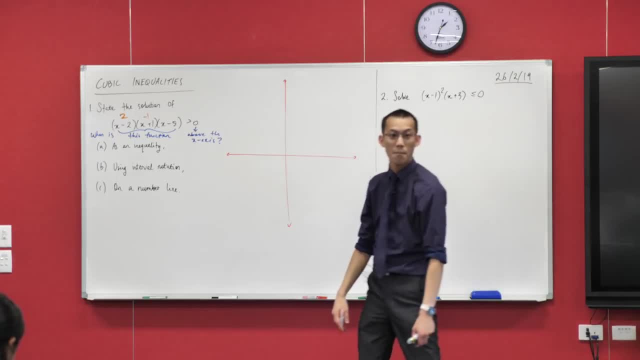 So I have another x-intercept and my last one, of course, is positive five. Thank you very much. Okay, Now I'm going to go from there straight over to my Cartesian plane and I'm going to mark in those spots on the x-axis. 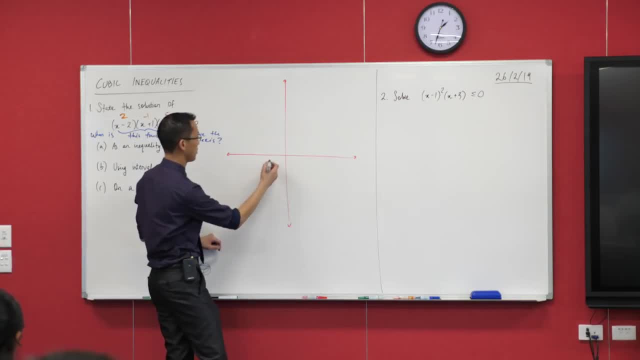 These guys are my x-intercepts I've got, let's see, here there's negative one, one, two. there's two, three, four, five. There we go: Negative one, two, five. So I've got my numbers on there that I've read off of here. okay. 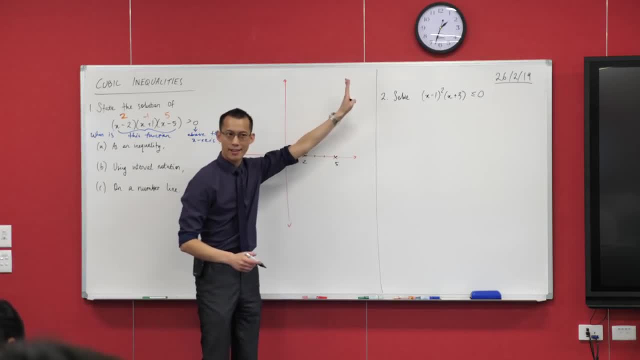 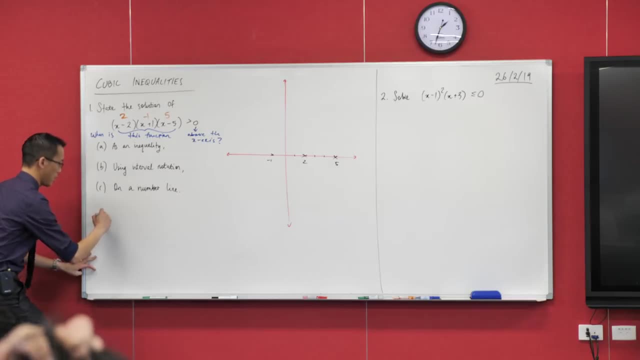 Now in the morning we wondered if you get these three intercepts right. there are a couple of different ways that the snake of our graph can weave its way through them right. So it's going to be either something that looks like this or something that looks like this: okay, 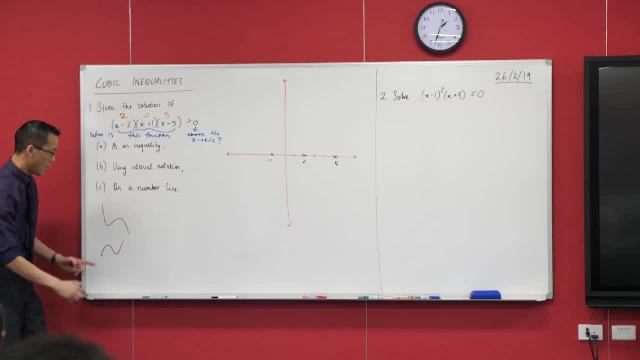 So what we did was we substituted some values in to see what would happen, okay, But in this case I'm just going to draw your attention to the fact that, were I to expand this whole thing, right and don't do it, I just want you to think if you did have a look at the x-cubed term. 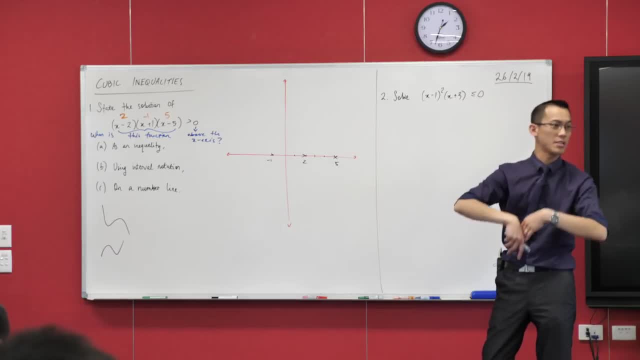 That's what makes this a cubic right. You're going to get some x-squares, you're going to get some x's, you're going to get a number at the end, but only one term will have an x-cubed in it. 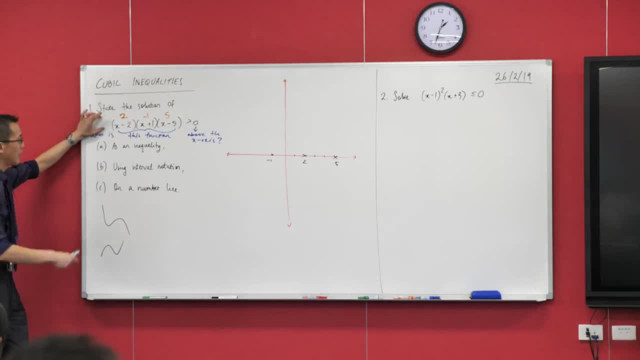 What would be the sign in front of the x-cubed? Would it be a plus or a minus? It's going to be positive. It's going to be positive. How could you tell? Because you haven't actually expanded it. What did you use to work it out? 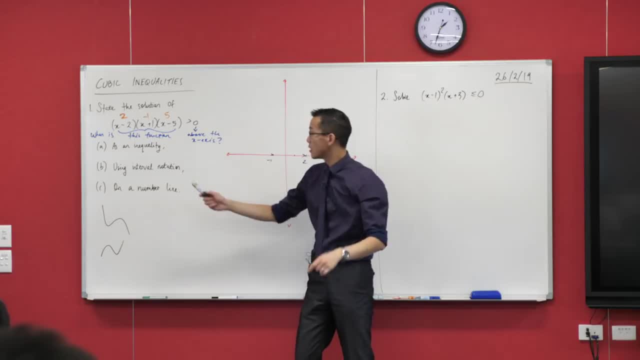 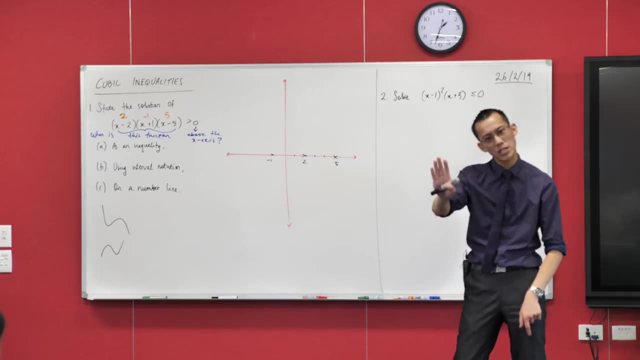 What do you reckon, Sean? I have no negative x. Yeah, very good. There are no negatives out in front of any of the x-pronumerals, right? So therefore, since you've got positive x, positive x, positive x, no matter what happens to the rest of it. 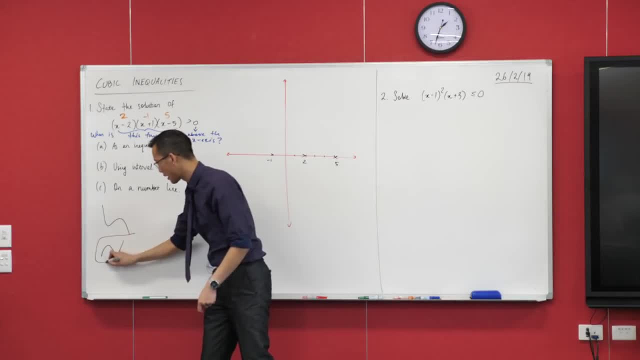 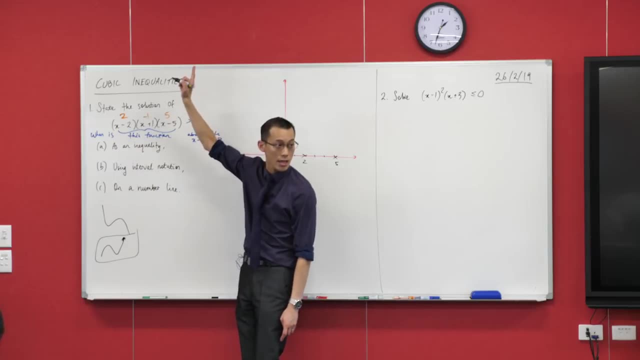 your x-cubed will be positive. That means you're going to get this guy here right, Because as you get bigger and bigger values of x, it's going to get more and more positive. Do you see that, As opposed to this guy? 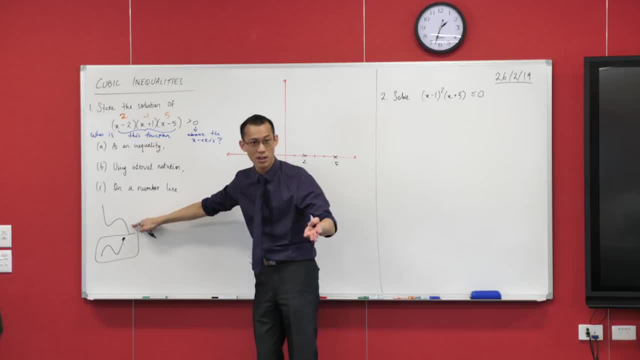 This guy here: as you get bigger and bigger values of x, does it get more positive? No, it goes negative. No, Bingo, It goes even more negative. So this is negative x-cubed. this is positive x-cubed. 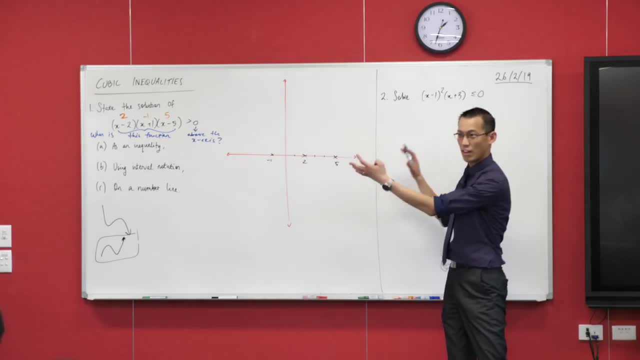 So I pretty much know all I need to know to now get a rough graph through here. It's going to go up right, Remember that- And then it's just going to kind of weave its way around like this. Now, at the moment I've got all the x-intercepts there and I just used that to get a general shape. 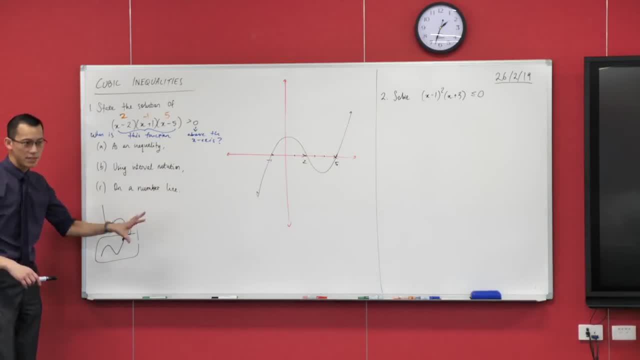 I hope you noticed. I haven't gotten the y-intercept yet and at the end of this, once we've finished answering the question, I'm going to ask you why I didn't bother to find it. But for now I'm going to go back to this blue writing: right? 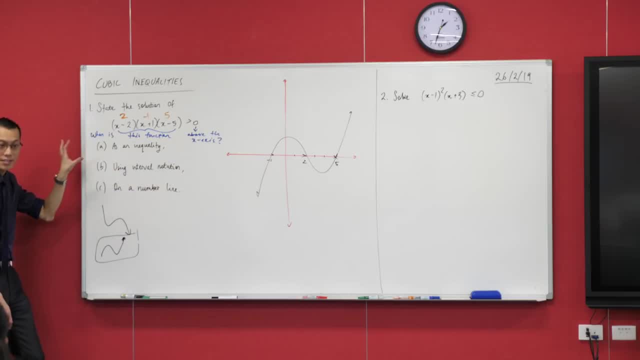 I now know what the function looks like. So the question is asking: when is that function above the x-axis? And you can kind of see those portions, can't you? If you've got another colour, I'd love you to grab that out. 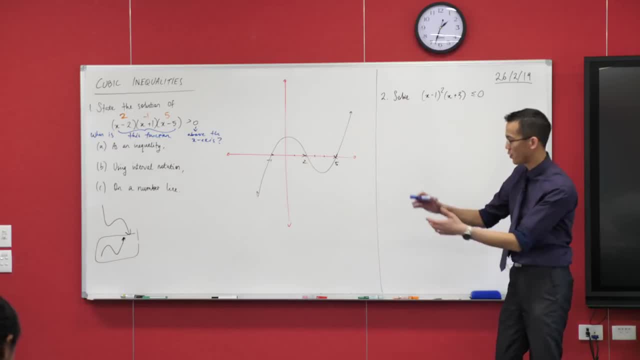 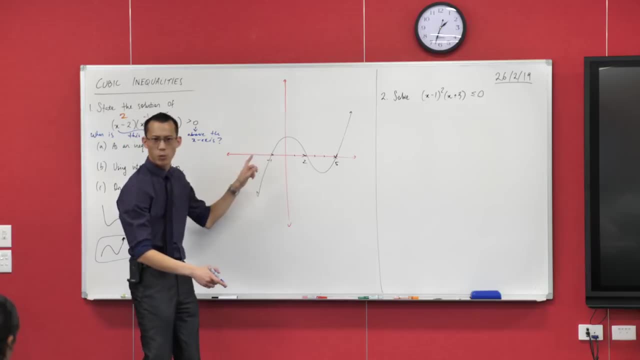 and whichever way you like, let's highlight the sections of this graph that are above the axis. Can anyone tell me where does the first section begin? Yeah, this, which dip were you drawn to Between where and where This top bit? This guy here Or this guy here? 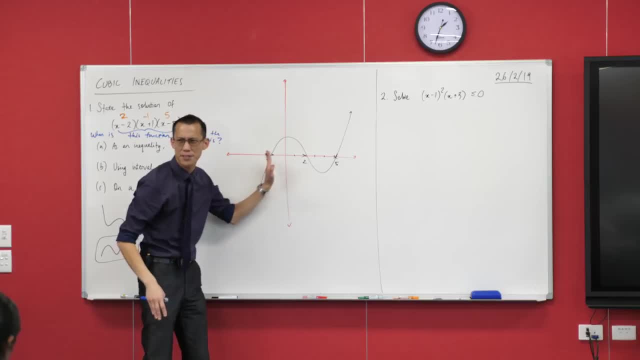 This one here is where we start, Okay, so I'm kind of going to go from left to right. So, like Sarain did, I'm going to start at this section here And I'm just going to mark it in with another colour, just so I can see it. 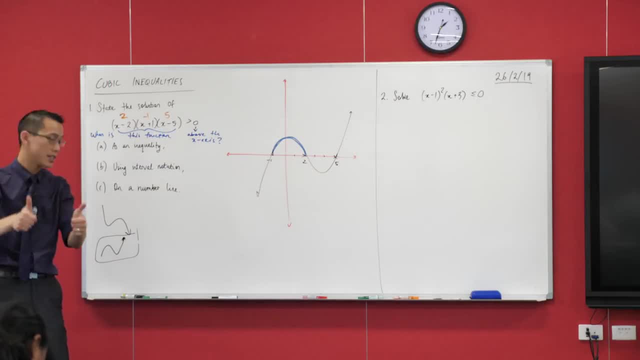 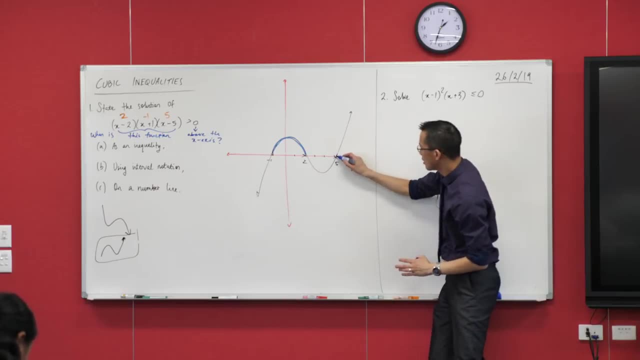 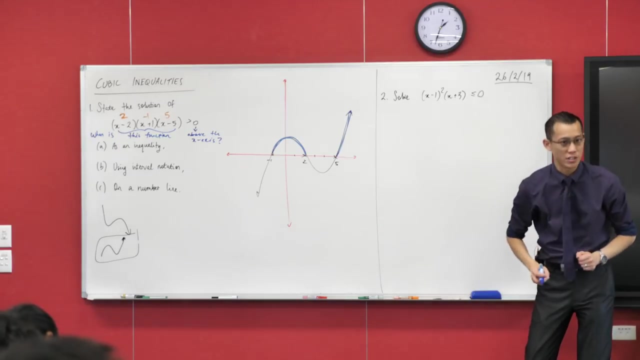 That part is clearly above the axis, So it agrees with what the question is asking. I do, of course, have another section. Where is it? Yeah, over this part here? So this is all above the x-axis. Above, y equals 0, which is because this is a y-axis and this is an x-axis. 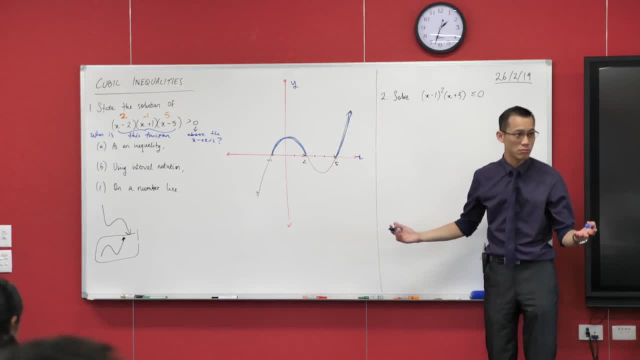 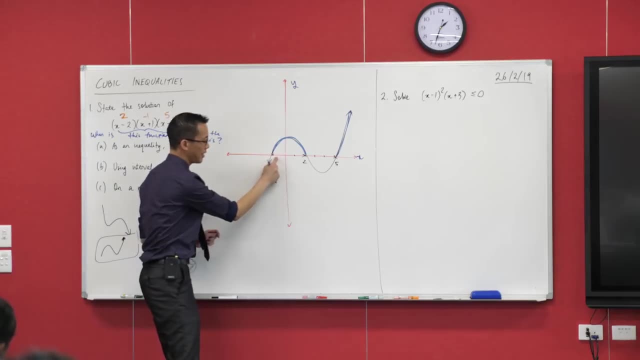 So these are the parts I want. Have I got them all? I'm pretty happy with them. Okay, I've got a quick question for you. My blue shading: it begins and ends, then it begins and then it just keeps on going. 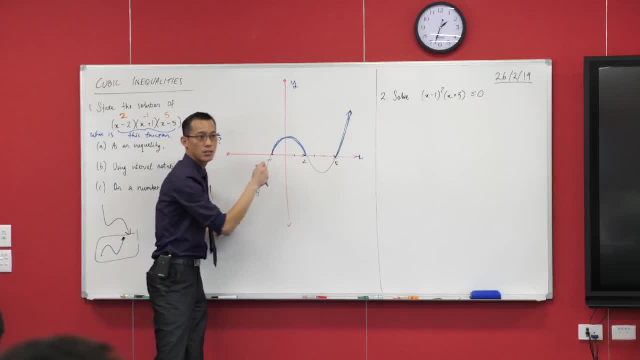 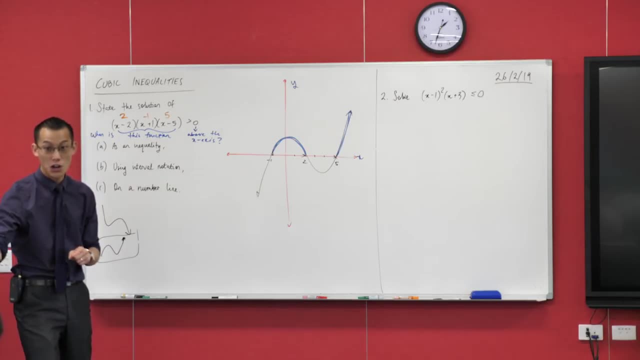 Am I allowed to include the actual beginning and end? No, exactly. actually, Now, it does depend on the question that you get. In this case, the answer is no. How could I tell? How could I tell, Yeah, see this guy here. 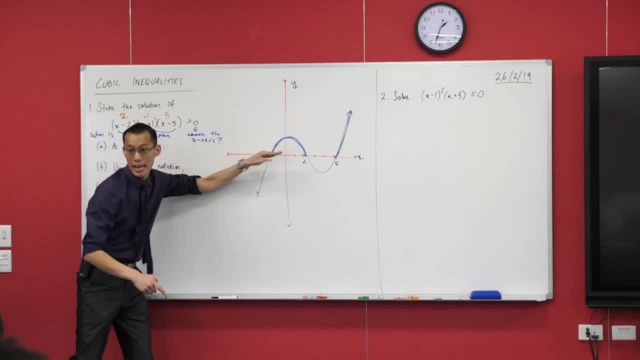 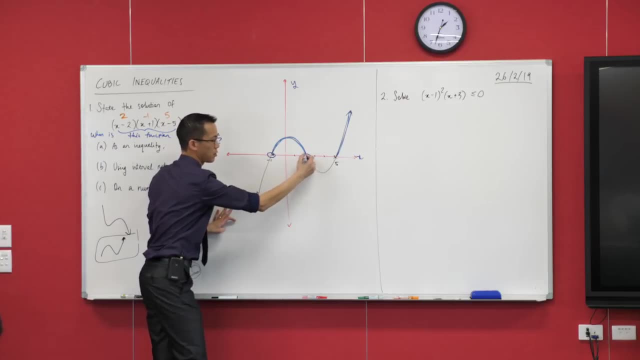 What this is saying is: I want you to not just be like on the axis. You have to be above the axis. You're not allowed to equal it. So these guys here I'm going to draw some big hollow circles like so Does that make sense? They're not included. 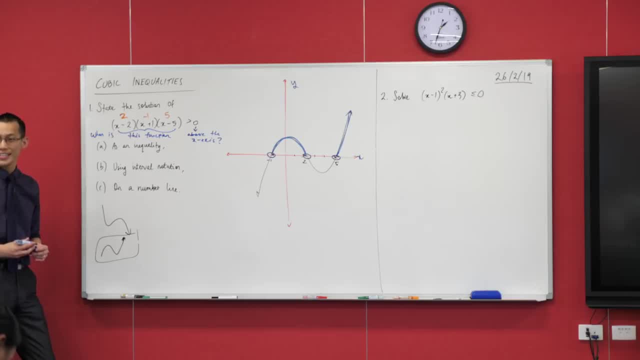 Alright, now, at this point, the graph has served its purpose. I've worked out when the function is above the x-axis, so I'm ready to answer these three questions and state this blue thing in the terms that they've asked for. okay. 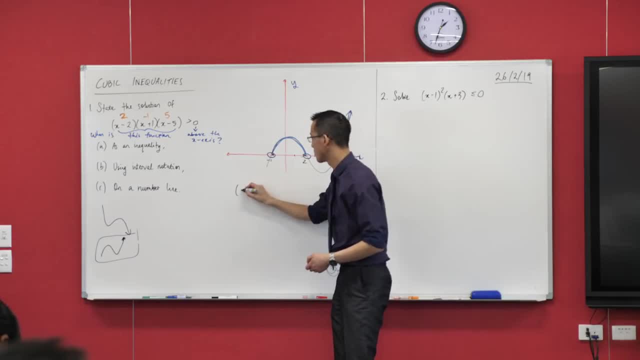 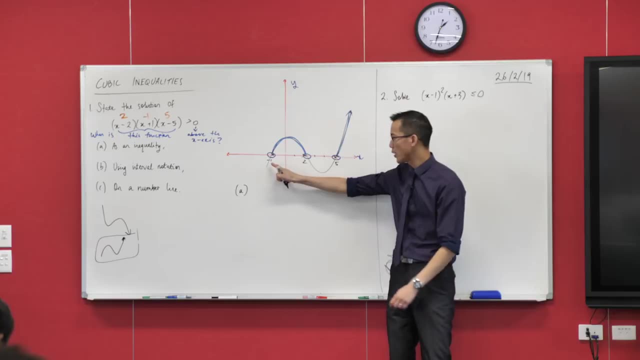 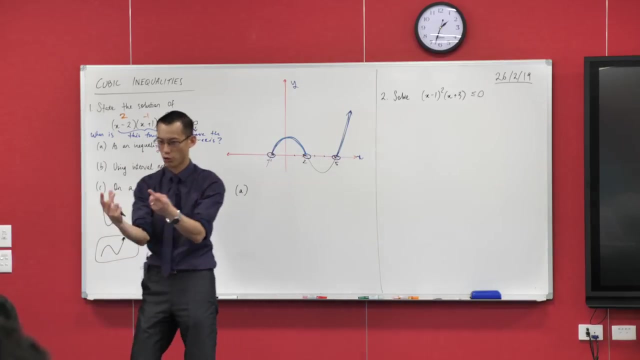 Well, that I've asked for. So here we go, Part A As an inequality. So I've got this part here And again. this is looking at what you did yesterday. Between negative one and two, We can write this section in one fell swoop with just a single sort of grouped inequality. 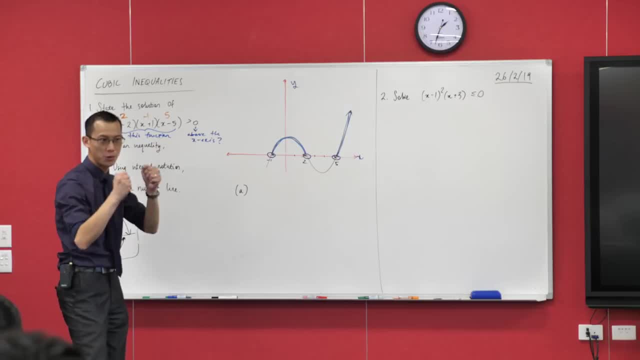 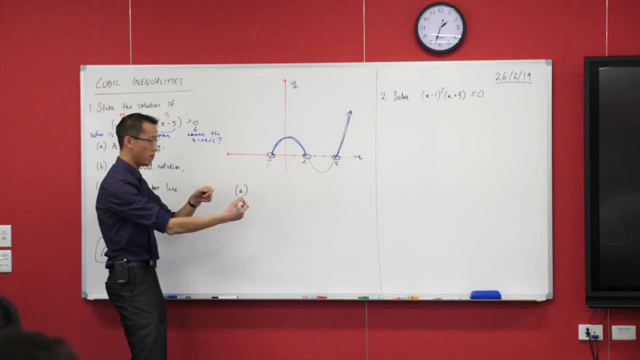 Can anyone tell me how am I going to write this? Hold that thought. Rishan, You've had some good inputs already today. Can someone else help me out? Hmm, Yeah, go ahead. Negative one greater than No less than. 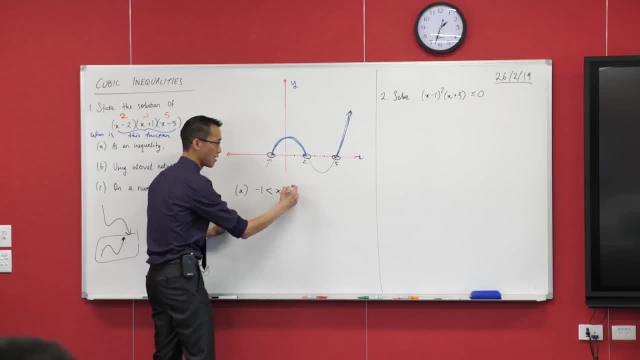 Less than X. greater than Now. before I write this next part, right, I want to be between here and here. Yeah, So in other words, that's greater than negative one Like zero's okay, Half's okay.